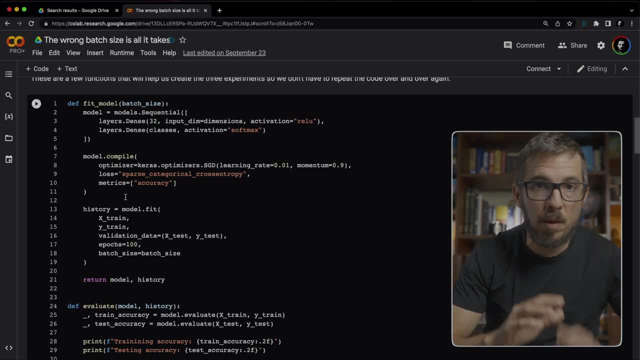 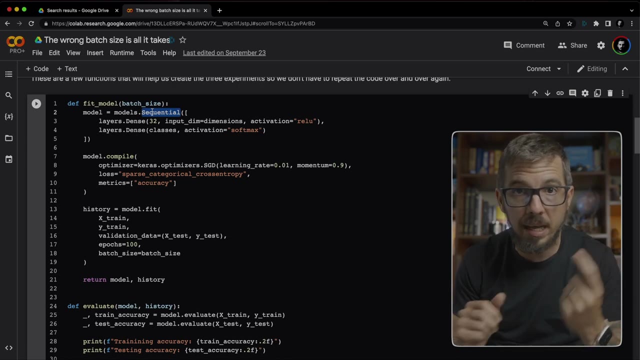 After creating that dataset. I'm defining here a couple of functions that I'm going to use on all three experiments. The first function, fake model, receives the batch size that I'm going to be experimenting with. It creates a very simple neural network with a couple of layers, one hidden layers. 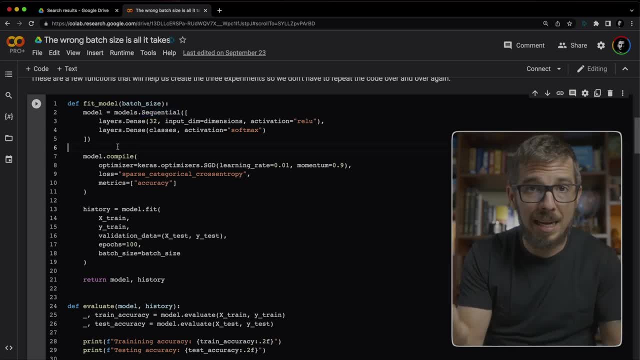 with 32 neurons And then I'm going to create a very simple neural network with a couple of layers, 32 neurons and the output layer. Then I'm compiling the model with gradient descent and finally I'm fitting that model Very simple, fitting on the training set. 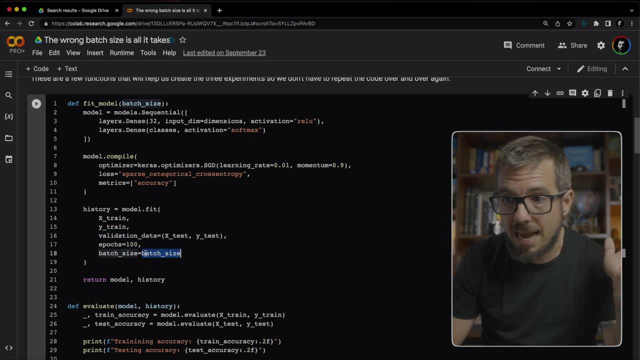 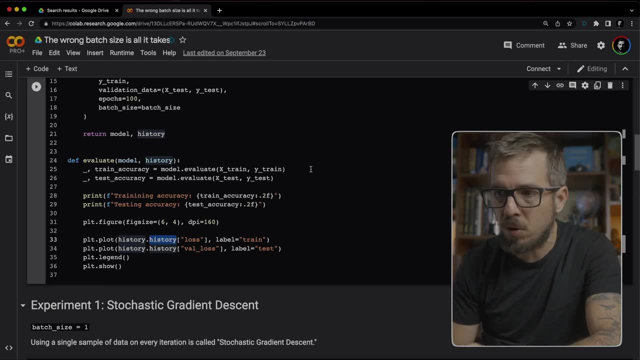 then i'm gonna be validating this model on the test set And notice that for the batch size I'm using the argument that I'm passing to the function Evaluate is very, very simple. First I'm evaluating the model on both the training and the testing set so we can print the accuracy. 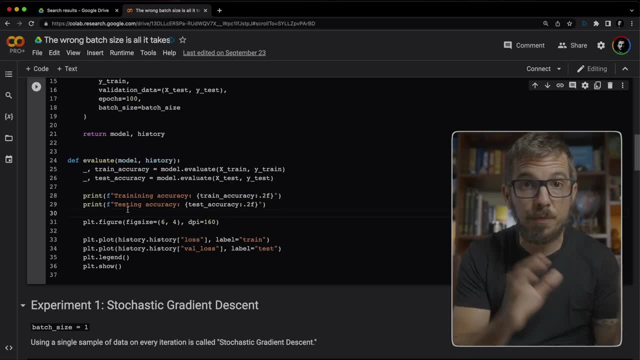 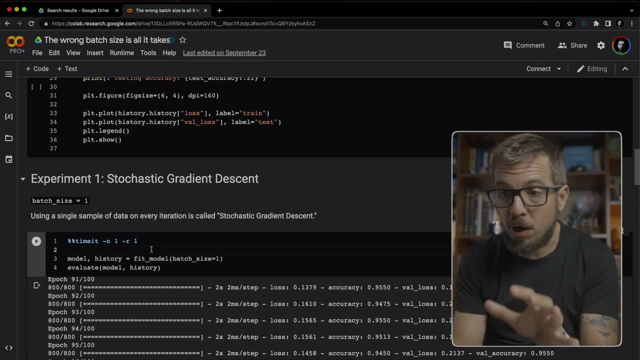 of the model And, finally, I'm plotting the losses from the training and testing processes. With all of these in place, we can start looking at the first experiment. This experiment uses a single sample, And whenever we use a single sample from the training dataset, we call it stochastic gradient descent, In case you 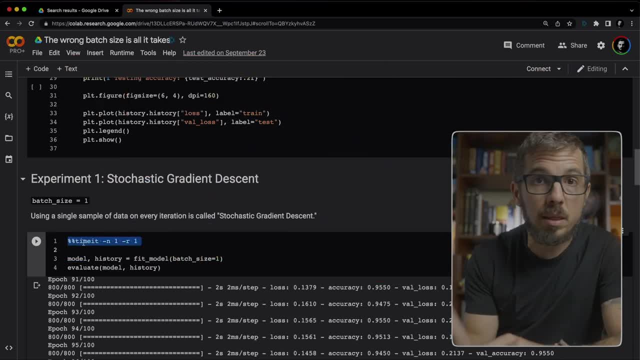 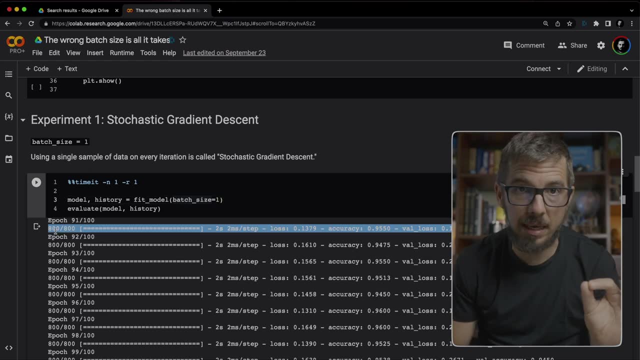 don't know what this line does. it allows me to compute how long this cell takes to run. Here I want you to focus on a few things. First, notice this 800 here. That's the number of times the algorithm computes the loss and updates the model's weights during backpropagation. 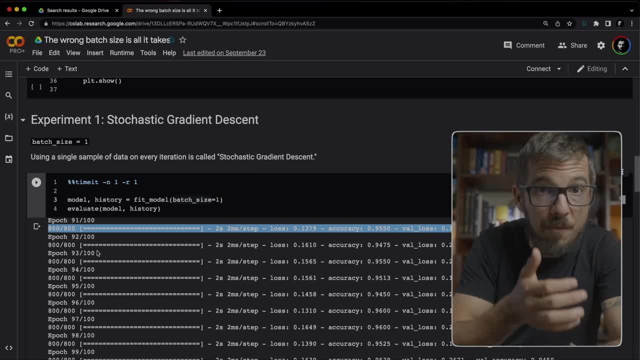 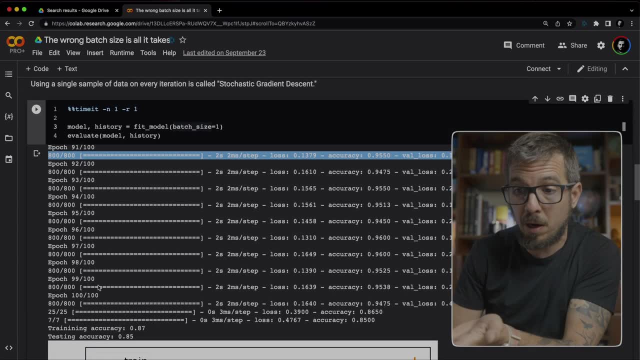 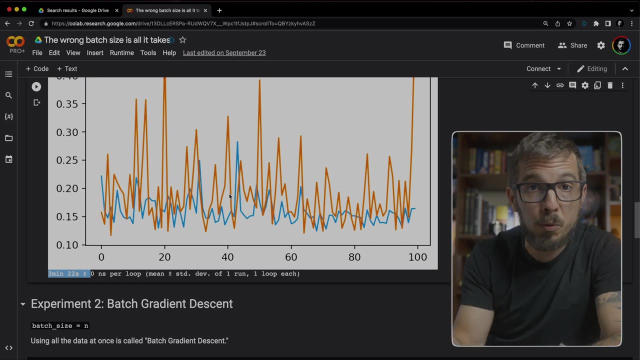 800 times. And it's 800 because we have a hundred training samples and we're using one sample per batch, And this, of course, means that this experiment takes a long time to complete: 3 minutes and 22 seconds, Having to compute the weights of the model. so many. 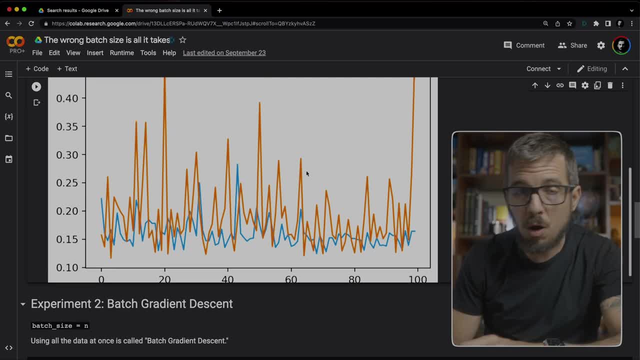 times is very, very computational intensive. Okay, let's get started. Let's get started. Okay, let's get started. Okay, let's get started. Now I want you to look at this chart. It's crazy. You definitely don't want that much. 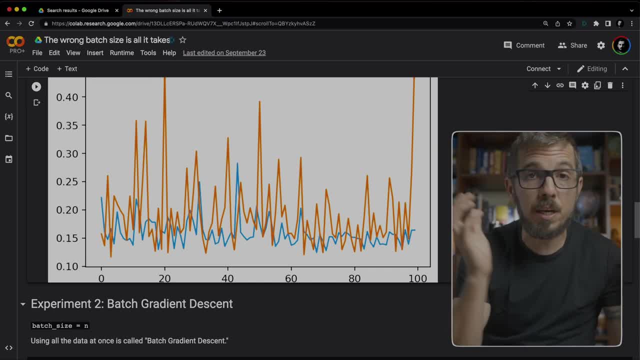 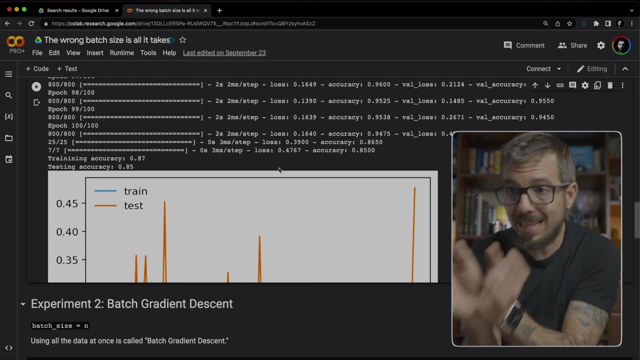 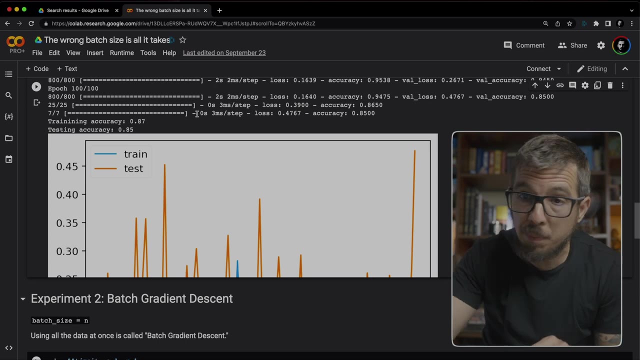 noise in your losses. The reason this is happening is because we're updating the loss for every single training sample. Finally, the accuracy of this model is in the high 80s. It's not great, to be honest, but there is something even more interesting If I run this experiment. 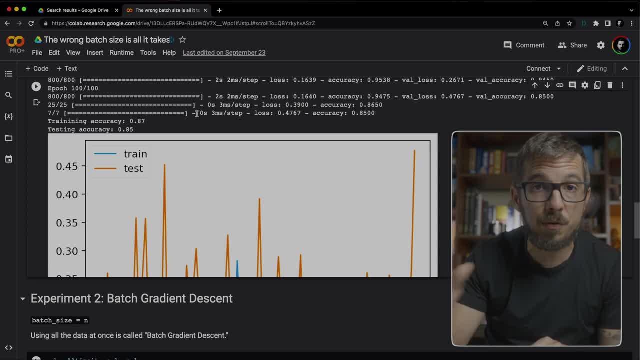 again, the results could look very, very different: Much better accuracy or worse, I just don't know. And this happens Because all of that noise, You see, the loss keeps jumping and it's very hard for the algorithm to settle on a good solution. Even if it reaches the global minimum, it might just jump right. 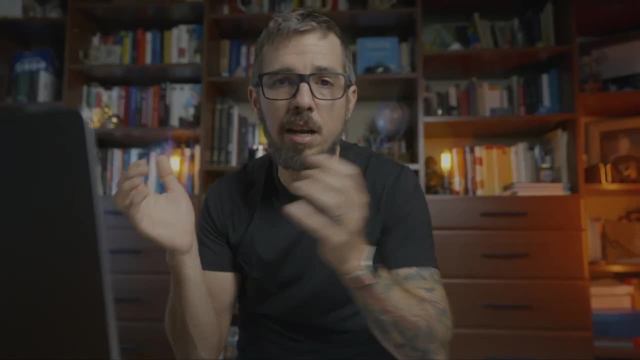 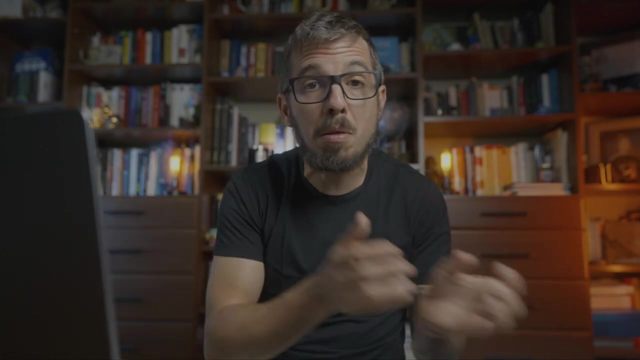 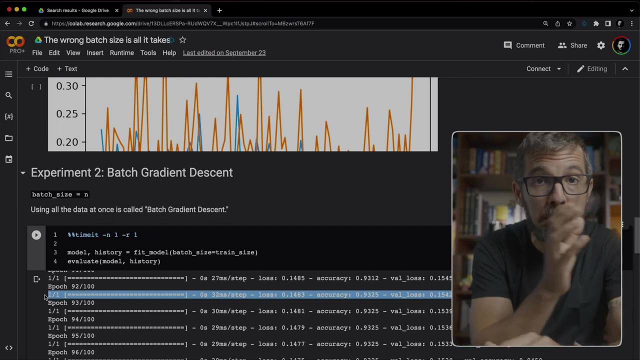 out of it. It's just too noisy. Let's look at the second experiment, And this time I'm going to use the entire training set as the back size. Using all of the data at once is called batch gradient descent. Notice that here it says 1 instead of 800.. We are now updating the models'. 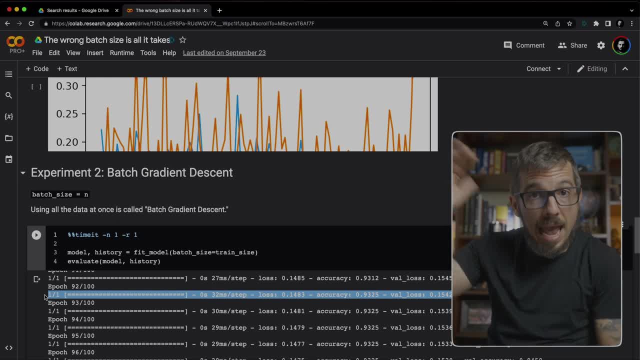 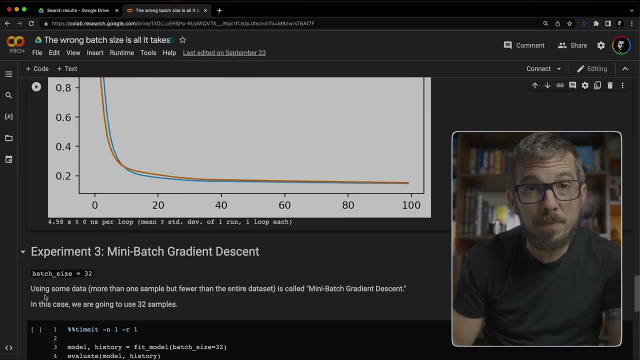 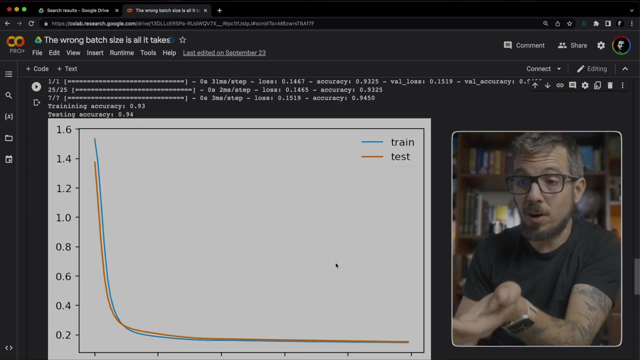 weights once during every epoch. So we went from 800 updates down to a single update. So of course, this model is going to run really, really fast: 4.58 seconds. Compare that with the 3 minutes and 22 seconds from before And look at the noise on this chart. It's none, It's zero noise. The accuracy: 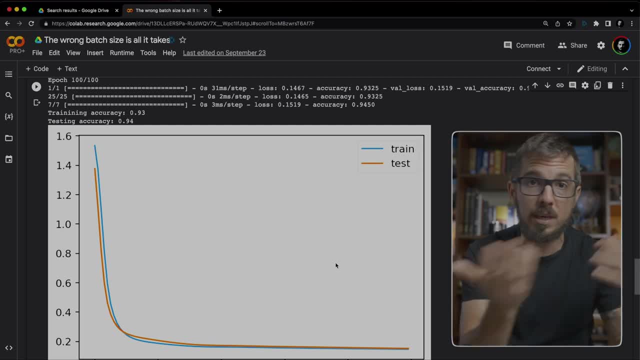 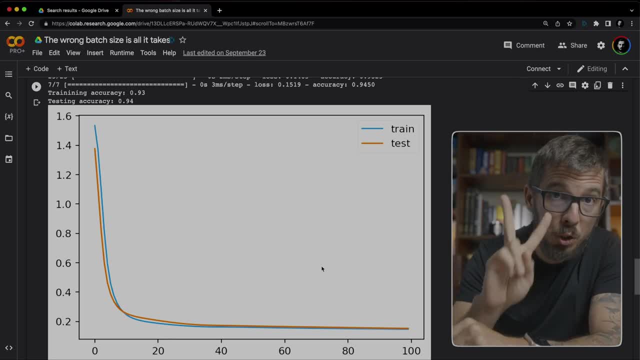 going to have to wait a little bit longer for this. So we're going to have to wait a little bit longer for this. So we're big problem that doesn't show here. actually two problems. first, this is a toy data set so we can easily fit the entire data set in memory. so we can compute the loss during every iteration, but in most. 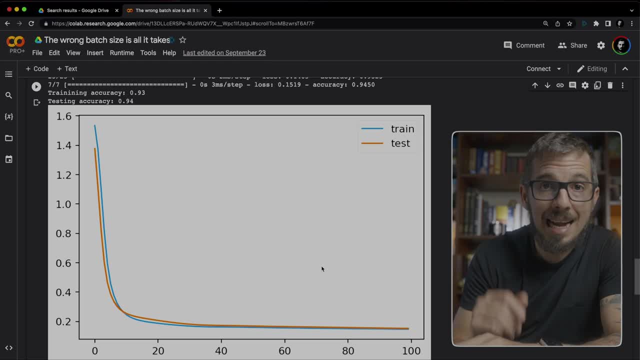 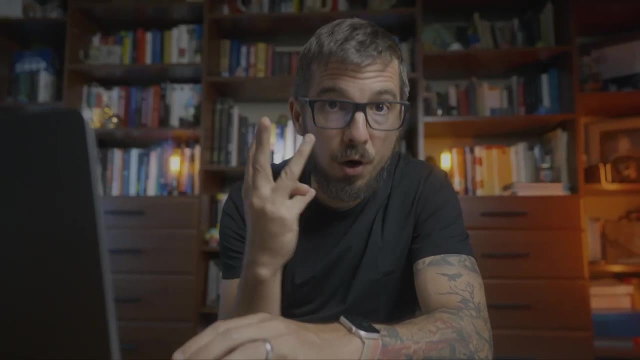 real applications. forget about it. you won't be able to do that. and second, that lack of noise can get us stuck in local minimum, just like too much noise will get the model jumping around. no noise will get you stuck. we need something better. so let's look at the third experiment. 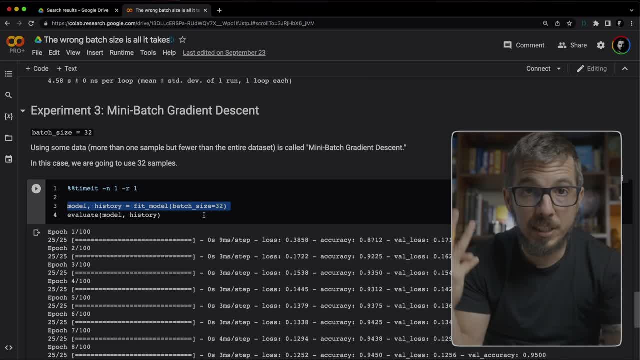 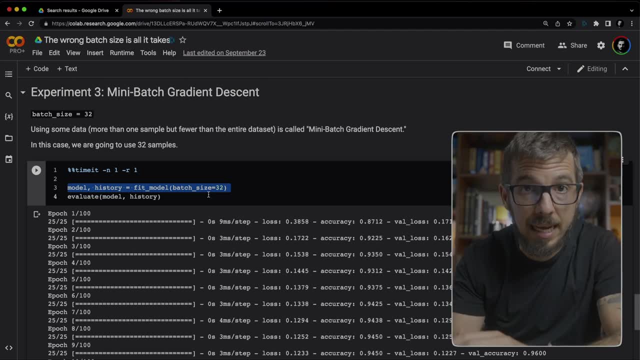 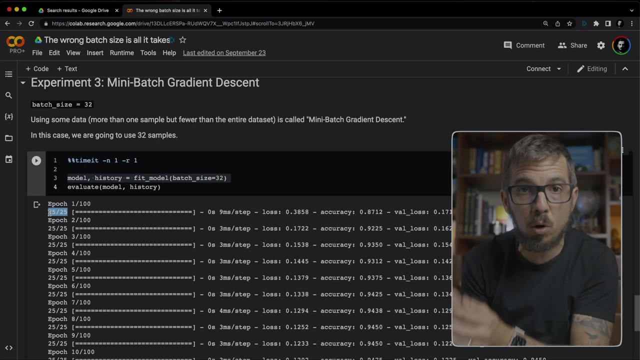 here i'm using 32 sample, 32 samples for my batch size, using a few samples- more than one, but fewer than the entire training set is called mini batch gradient descent. now this 25 here tells us that we are updating the model's weights 25 times during every epoch. now this, of course, runs pretty fast.